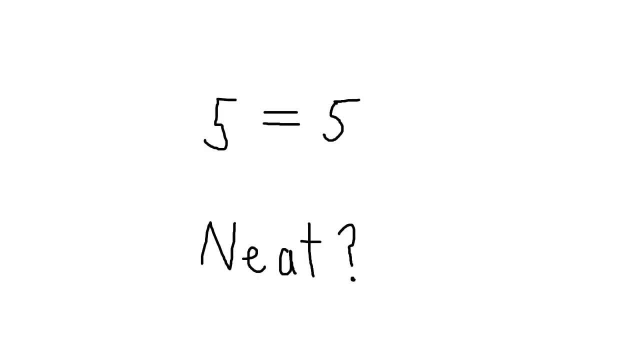 This introduces the concept of the equal sign, which implies that the terms on the left side side of the equal sign are equivalent in value to the terms on the right side of the equal sign. 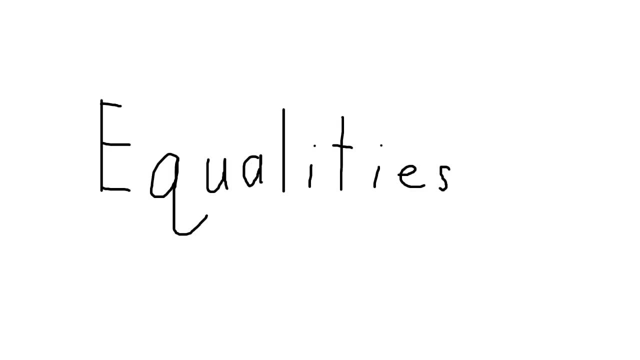 The equal sign also introduces the next concept, equalities. For example, variables may not necessarily start isolated. 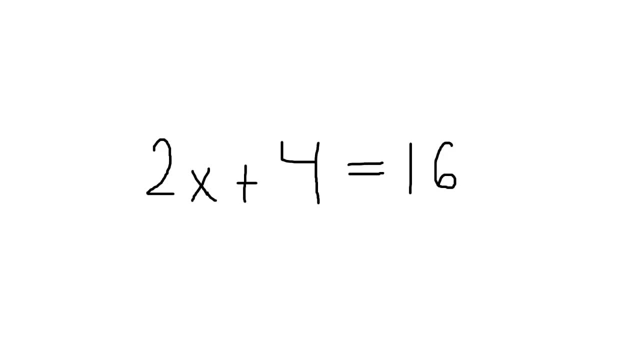 You may have an equality that looks like this, 2x plus 4 equals 16. Since we wanted to know what x is, we need to reverse engineer this equality, and by that I mean we literally need to solve the problem by using order of operations in reverse. 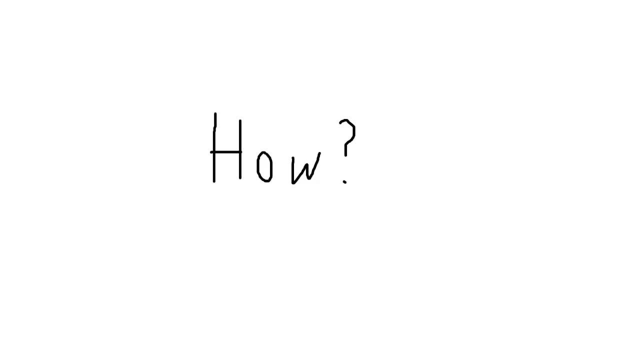 Now the big question, how do we do that? Well let's look at an obvious equality, 4 equals 4. 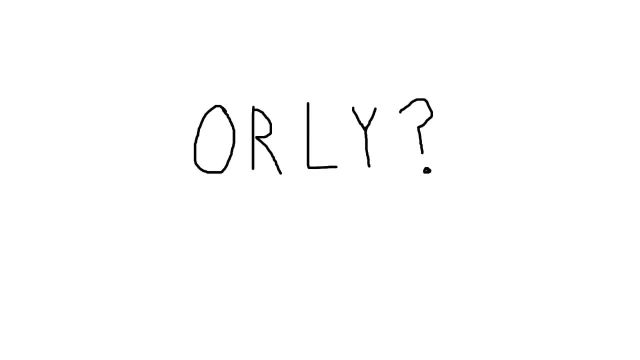 This is a true statement. If we add, subtract, multiply, or divide any number from both sides of this equation, we still get a true statement. 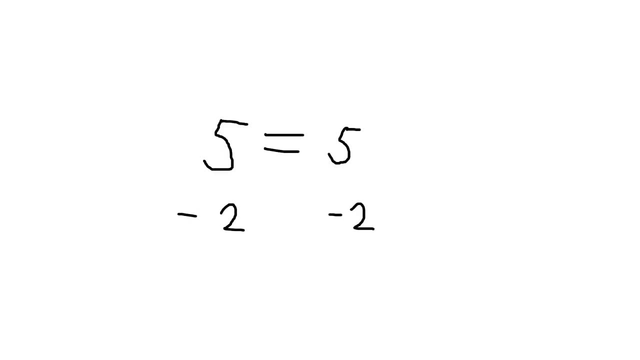 4 is still equal to 4, 5 is still equal to 5, 3 is still equal to 3, 6 is still equal to 6, and 2 is still equal to 2. 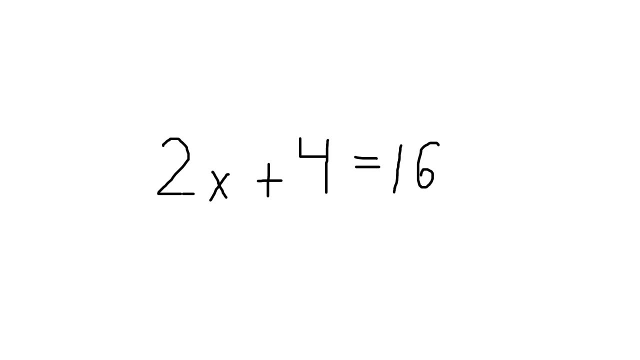 So going back to the problem that we had before, we solve it by using order of operations in reverse. Then adding, subtracting, multiplying, or dividing values to both sides of the equation to make effectively nothing different. 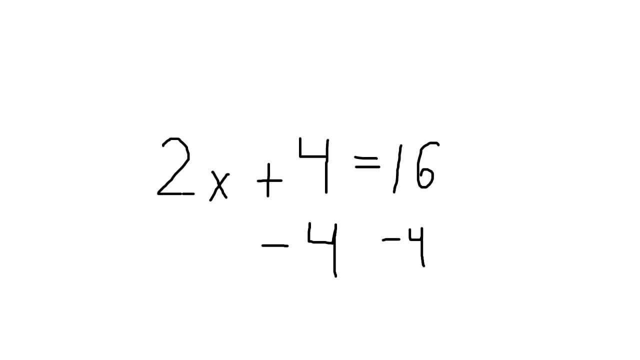 If we subtract 4 from both sides of this equation, we get 2x equals 12. Then if we divide both sides of the equation by 2, we get x equals 6. 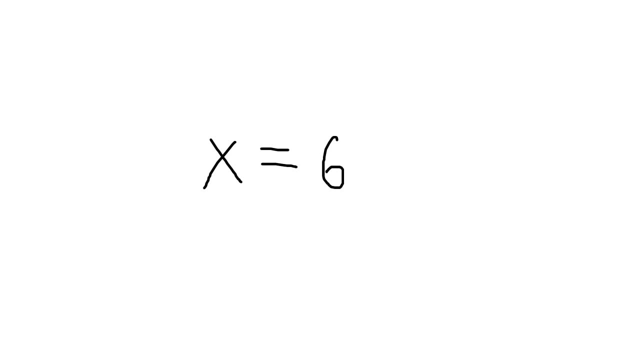 Then if we look really carefully, we can see what x is. 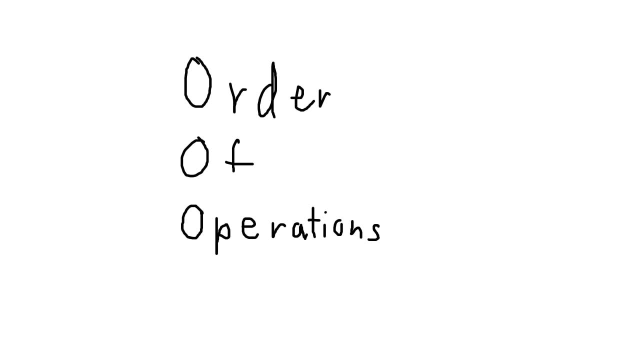 Don't worry, order of operations is really easy to remember if you just remember this expression. 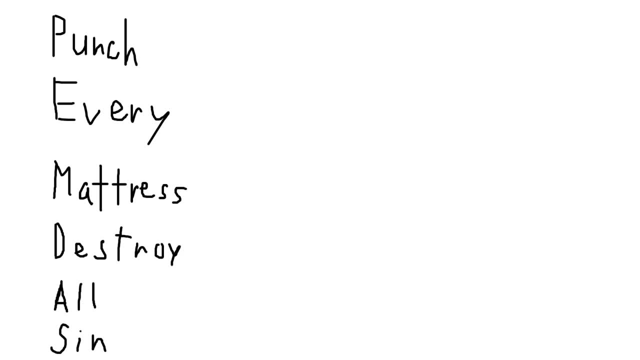 Punch every mattress. Destroy all sin. Or in this case, when it's in reverse, sin all destroy, mattress every punch. Or my personal favorite, nesla elrshshshshsh. 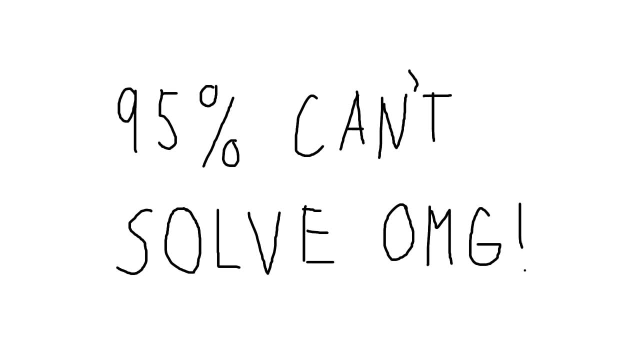 So now, when you see those posts from 2010 that say 95% of people get this question wrong, 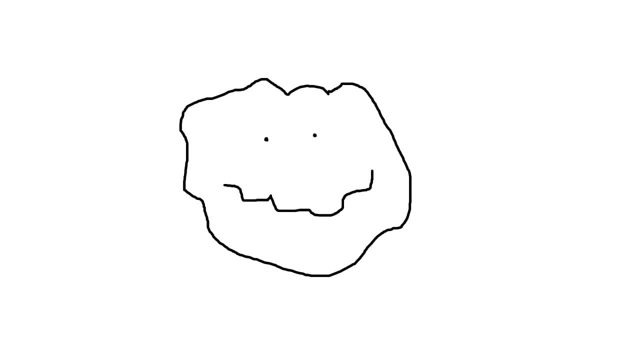 you can prove that you're in the top 5% by showing a basic competency in 8th grade algebra. In addition to equalities, there's also inequalities, like this one, and the way to solve inequalities is very similar to solving inequalities.